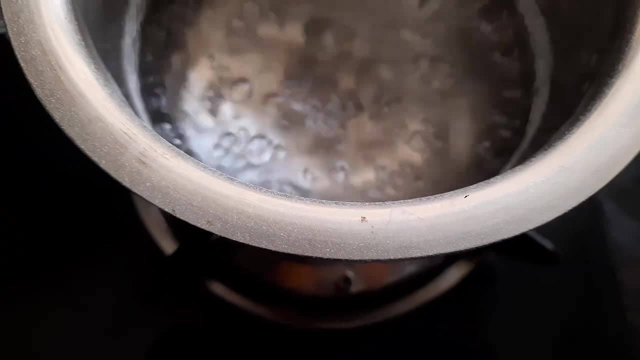 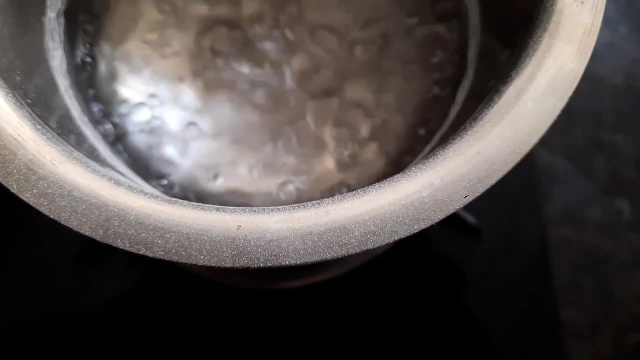 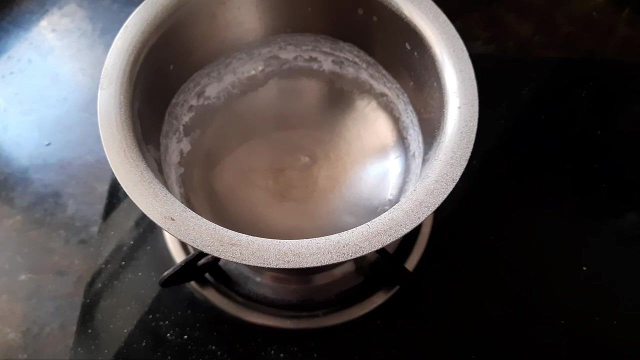 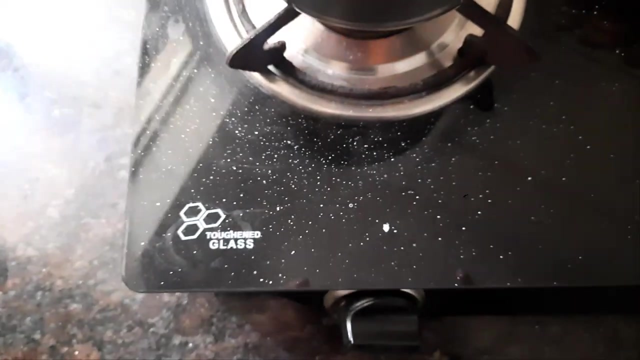 deposited on the sides of the container and also on the top of the container, Just like how you see in front of you. Most of the water has been boiled and see the salt that has been deposited on the sides of the container and also what you see around the container. This is also salt. So the salt that 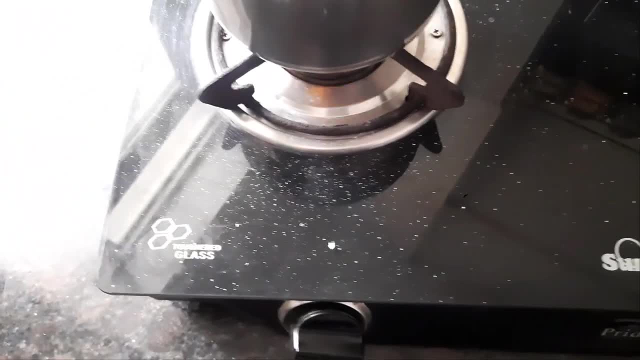 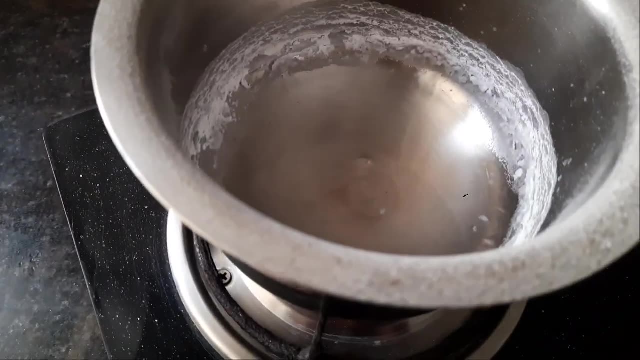 you dissolved. this is the same salt that you see in front of you outside the container and also deposited around the container. All right, at this point I wanted to think about whether this is a physical change or a chemical change. So turns out that this is a physical change. 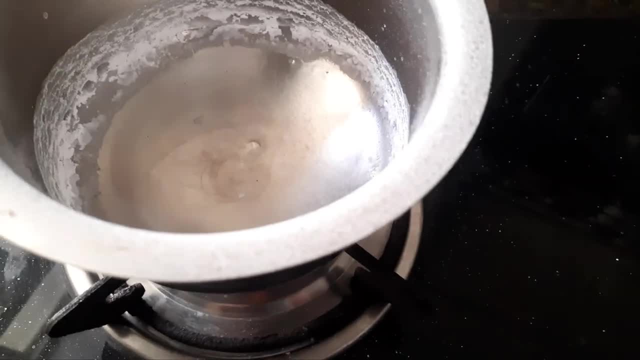 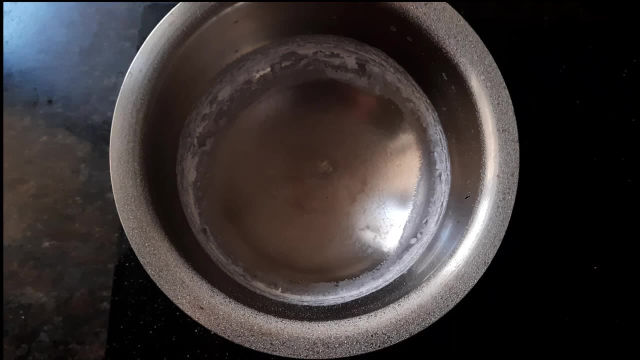 Because you started with salt and there was a process that happened and again you ended with salt. You dissolved the salt, then I vaporized the water and then again we got back the salt that we started with. So no new substance was formed and also this process was reversible. 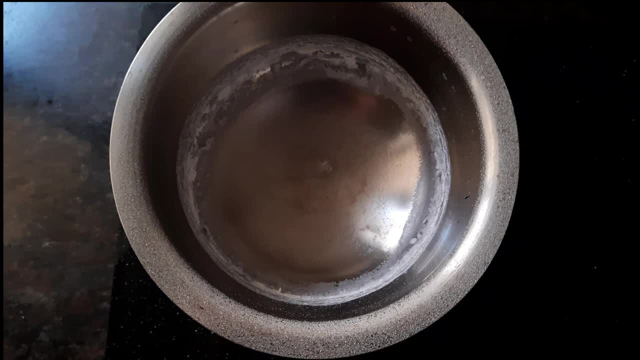 We could obtain the salt that we started from, So this was a physical change. So dissolving salt in water is a physical change, because we can get back the salt that we started from and no new natural substance is formed. So this is a physical change. 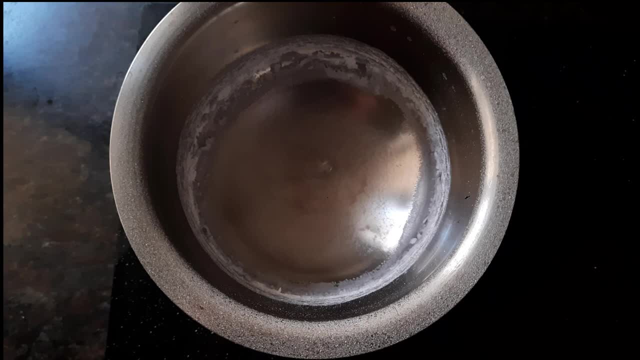 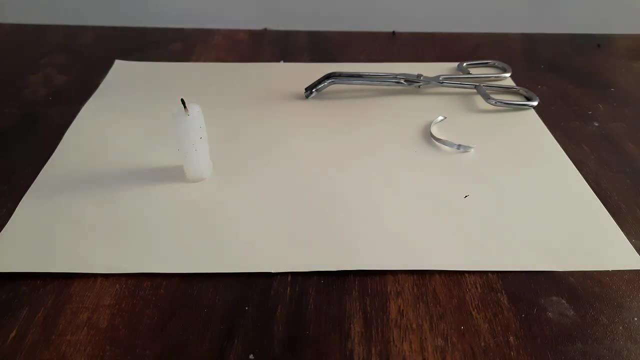 Nothing, nothing new is formed. All right, let's look at one more case Now over here. I have a candle. I have a lighter. I can use this to light up the candle. I have a magnesium ribbon and a pair of tongs. 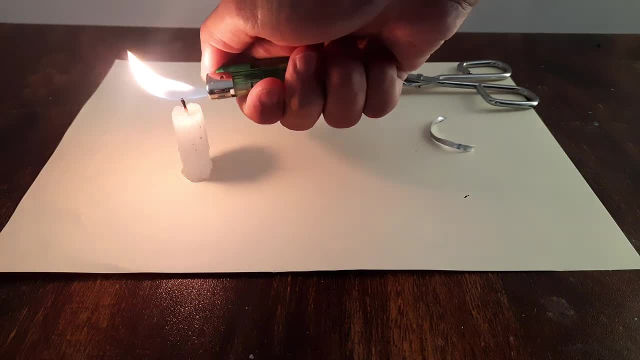 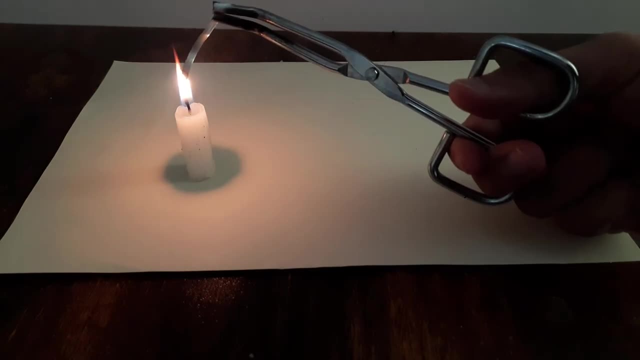 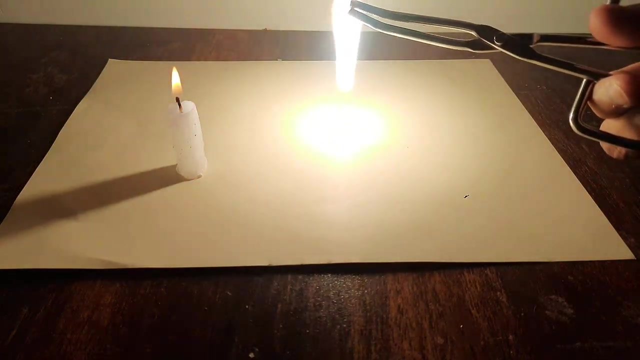 So I will light up this candle and I will try and burn this magnesium ribbon And I want you to notice what happens. Oh, look at this. Look at how bright, how bright the magnesium ribbon burns. The candle is not even visible. 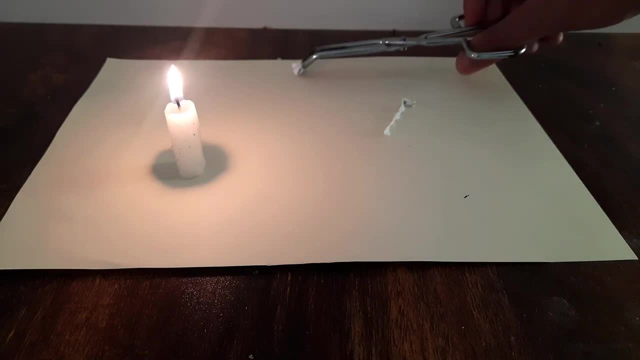 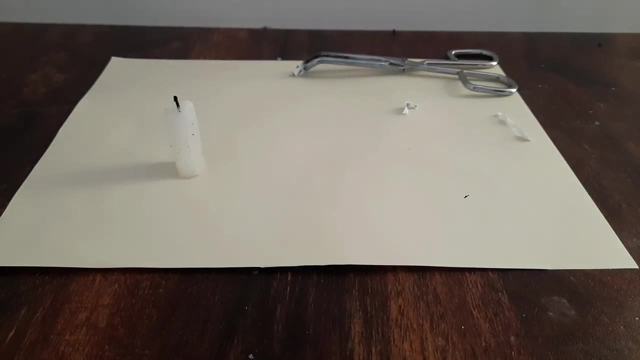 All right. So what sort of a change was this? Was this a physical change or a chemical change? Okay, so it turns out burning of magnesium is a chemical change, Because here, when magnesium reacts with oxygen- and it's reacting with oxygen in the presence of oxygen- it's not a chemical change. 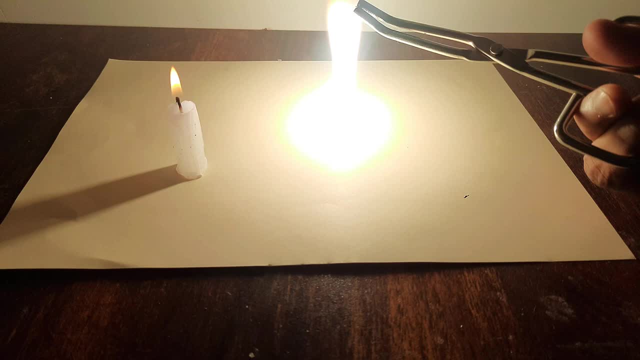 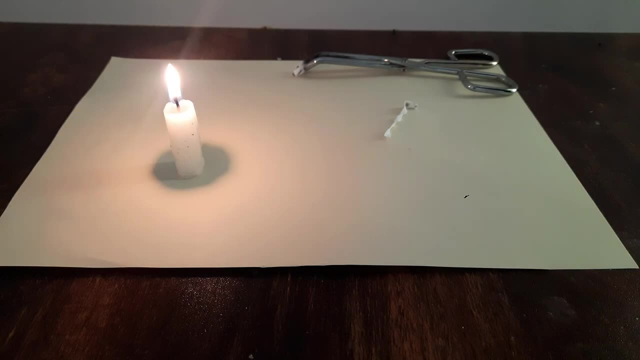 It's a chemical change. It's a chemical change because of so much heat. When that happens, new substance was formed. That was magnesium oxide, And you can't really go back from the burnt magnesium ribbon to the original magnesium ribbon that there was.